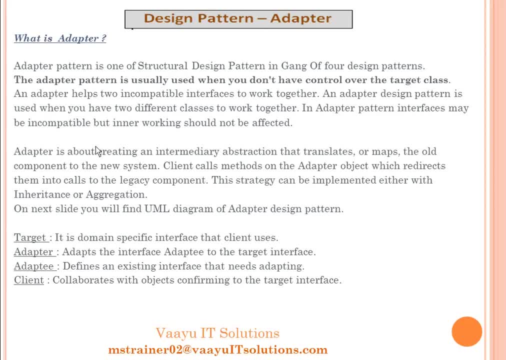 So what is adapter? Adapter pattern is one of structural design pattern in Gang of four design patterns. We have been discussing in our previous sessions that what is the Gang of four design patterns? Okay, So this adapter pattern is used when you don't have control over the target class. 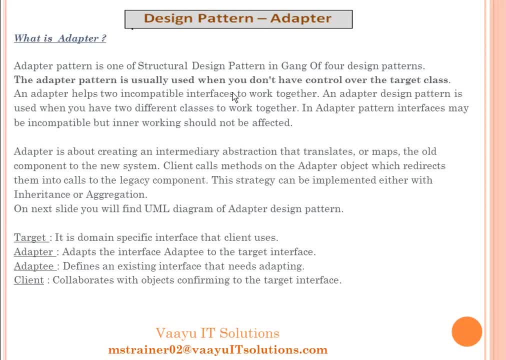 You have some target class on which you don't have control, Okay, But still you want to use it some way. Okay, So an adapter has two compatible interfaces to work together. Okay, An adapter design pattern is used when you have two different classes to work together. 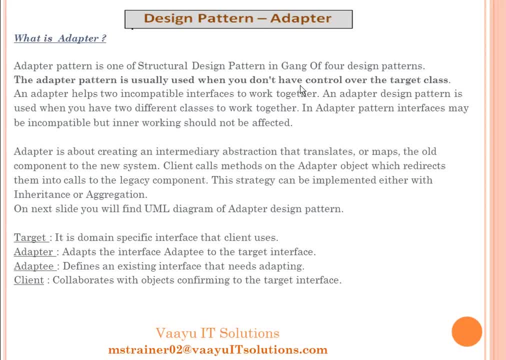 It is a project requirement that you have some classes or different classes, which has incomplete- Okay, So an adapter design pattern is used when you have two different classes, which has incompatible interfaces. Okay, And you want to use them? Okay, Let us take an example. like you have some component. 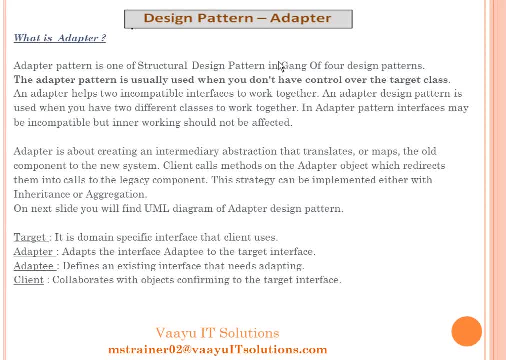 Like VVC component or XF component. So NET works this way. NET has provided some libraries that works as a wrapper over the component. Okay, We call the, we execute the method on those libraries, but actually it is hitting the dotnet component methods. Okay, so what is this after? do it translate or maps the old component to the new system? or you have some component that is that is incompatible with your existing system. 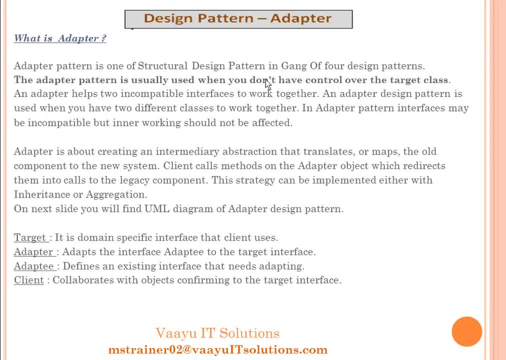 Okay, So we call methods on the after object, which redirects, calls to the legacy component. Okay, that is your adaptive. Okay, This strategy can be implemented either with inheritance or with aggregation. Okay, so now. now let us see the what is the after design pattern in the UML diagram. We have a target adapter and the adaptive. 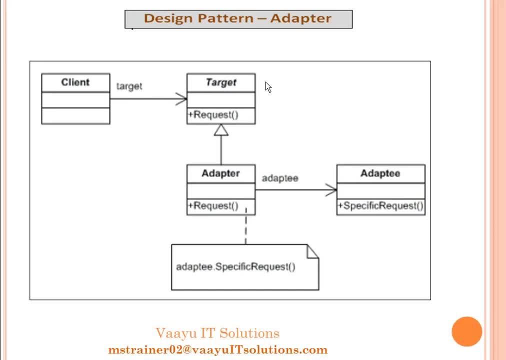 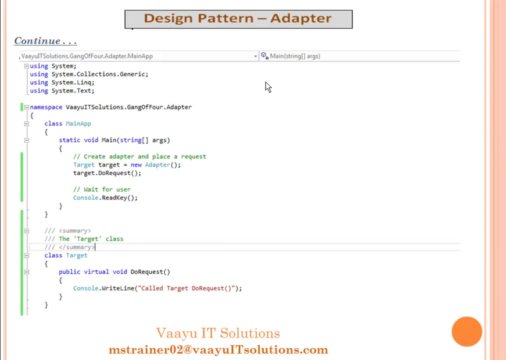 Adaptive has the method that will be executed by the adapter. Okay, and this is the target. We know what does the client do. Client will shoot some operational method for working, Okay. so we see that we have one target class, that is the virtual method. do request: Okay, and we have the adapter. that is inherited. 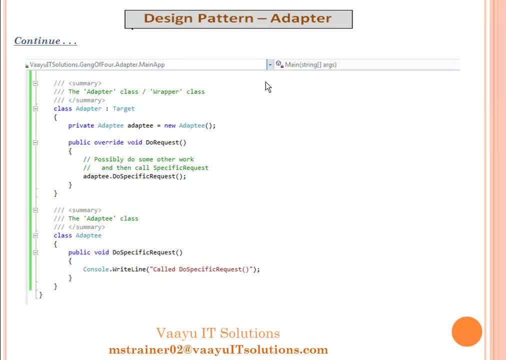 Executing the target class. Okay, and this adapter. we have the adaptive object. Okay, and this overridden method of the target class. I mean the target has a virtual and after is the direct class, So it is overriding. We are executing the adapter or do specific request method. 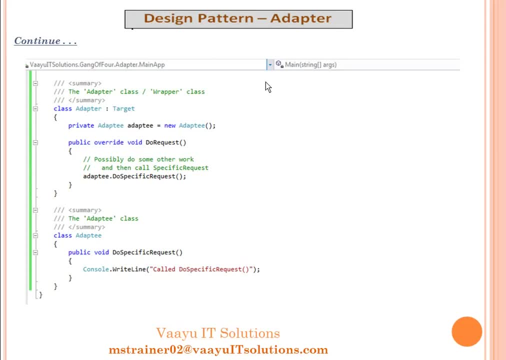 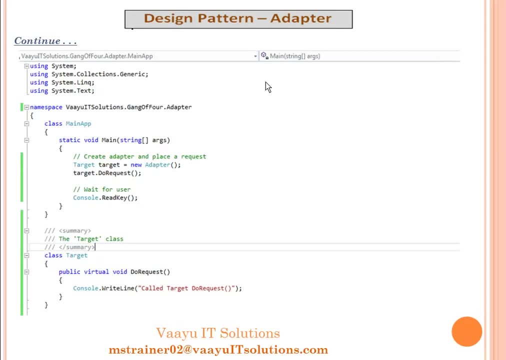 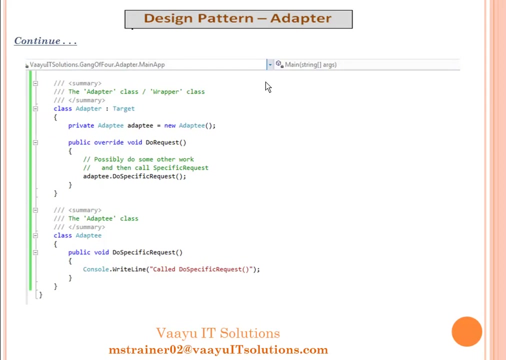 Okay, So we see that actually it is hitting the legacy component method. In the static void method we have a target target equals to new adapter, Okay, and we are hitting the target or do request. Then it will execute the direct class do request method. Then further it will execute the adaptive dot do specific request method. Okay. 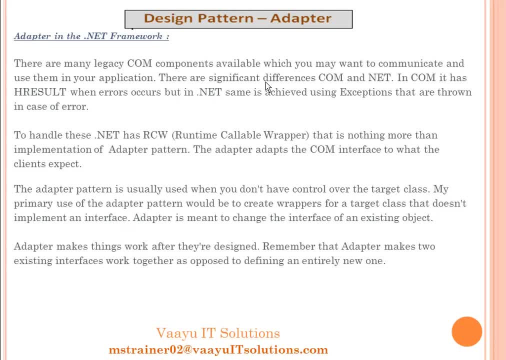 So we see that we use the after pattern when you want to or when you need to create some wrapper around your common interface. Okay. so we see in dot net we have the exceptions Right, But in the com we see that it has the edge result. Okay, so suppose you need to create some wrapper over com edge result. Then you want to do it in the exception Right. 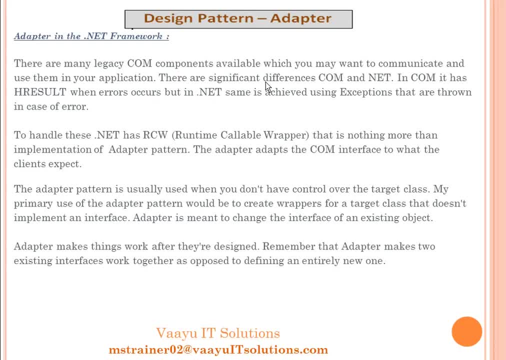 Exception way and you can do this. Okay, because of we don't have control over the com component, com interface. Okay, So we can say the after pattern is usually used when you don't have control over the target class. Okay, And you need to create wrappers for a target class. Okay, that doesn't implement the interface. So after is made to change the interface of an existing interface. Okay,